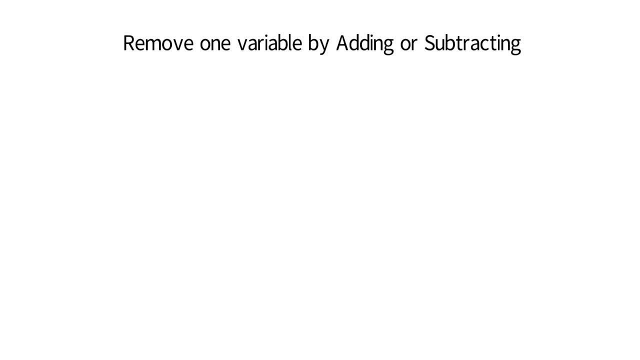 Let's look at an example to explain it. Solve the simultaneous equations: 4x plus 2y equals 15 and x minus 2y equals 5.. Let's call this equation. The first step is to choose the letter you want to eliminate. 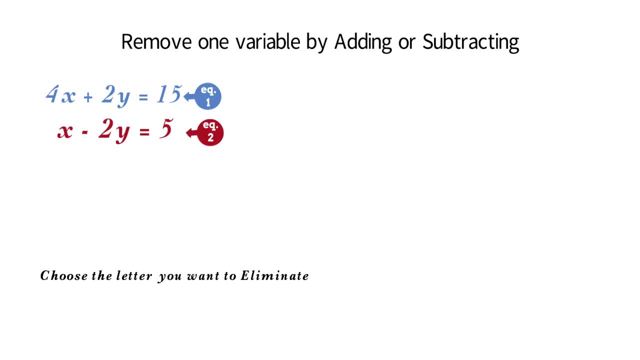 You can choose any of the letters, but if you have one with the same coefficient, it would be best to choose that one, because it will take care of step 2.. So here I will choose the y. Next, we want to make the coefficient the same. 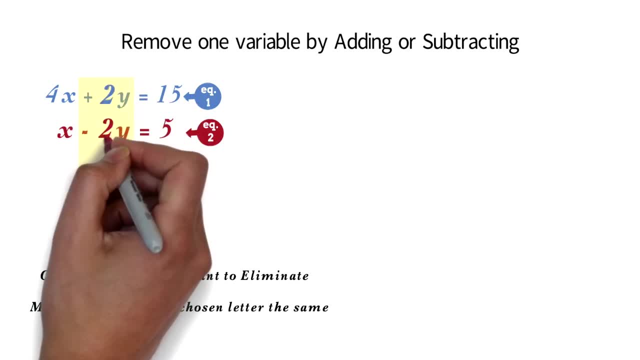 Because we chose y, which has the same coefficient, we will have to make the coefficient the same. If we choose the coefficient of 2 for both equation 1 and 2, there is nothing to do in this step. The next step is to eliminate the y values. 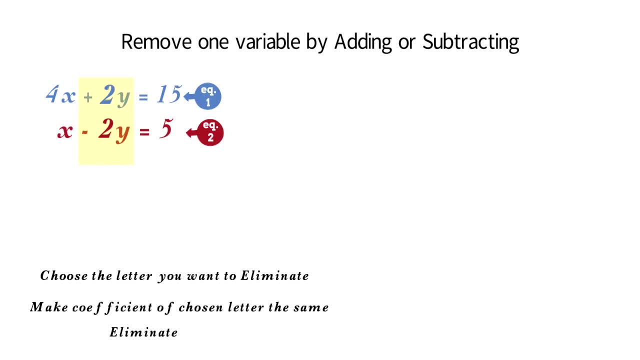 Since one is positive and the other is negative, we can add the two equations so that the y value will be 0.. 4x plus x will be 5x, 2y plus negative 2y will be 0. And 15 plus 5 will be 20.. 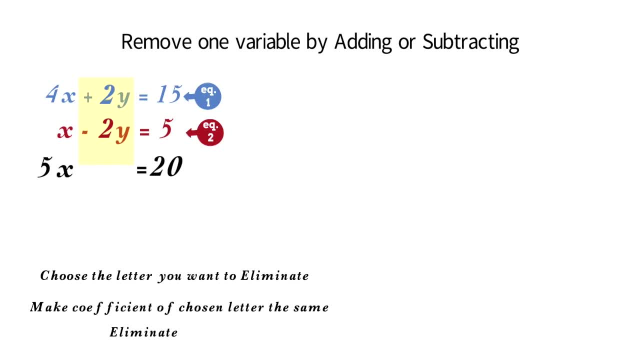 Now we can solve this one step. equation: 5x equals 20.. The 5 is multiplying, so we will divide both sides by 5.. The 5 cancels out 20 divided by 5.. 20 divided by 5 is 4.. 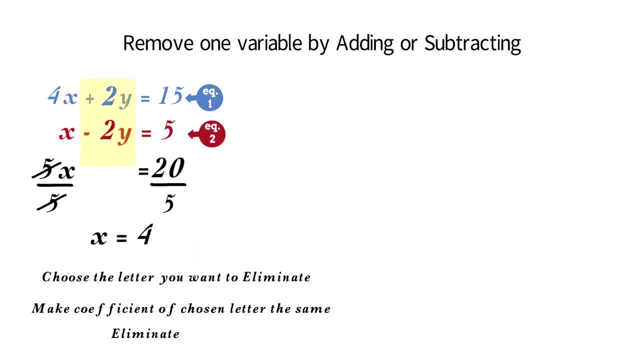 Therefore x equals 4.. Finally, we can replace the x by 4 in equation 1 or 2. to solve for y, I'm using equation 2.. We have 4 minus 2y equals 5. We have a two-step equation here. 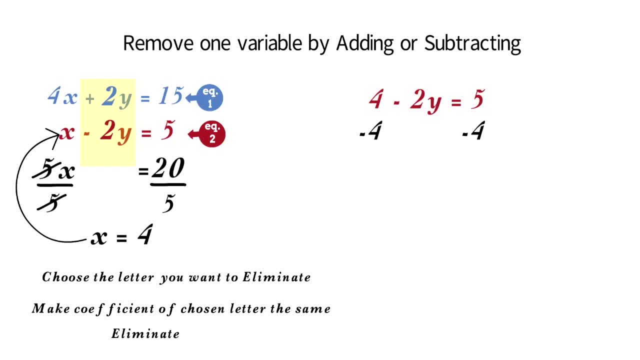 Subtract 4.. Subtract 4: from both sides, The 4 will cancel out. 5 minus 4 is 1.. So we have negative 2y equals 1.. Next we will divide both sides by negative 2. The negative 2 will cancel out. 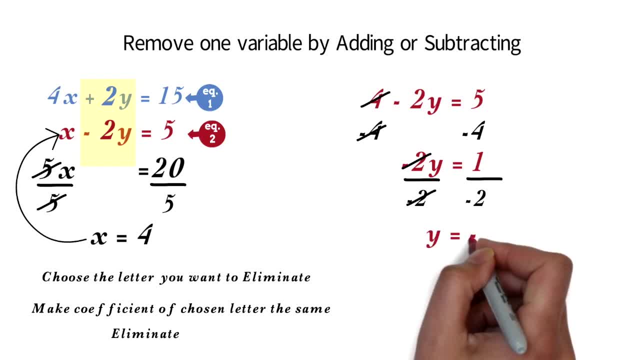 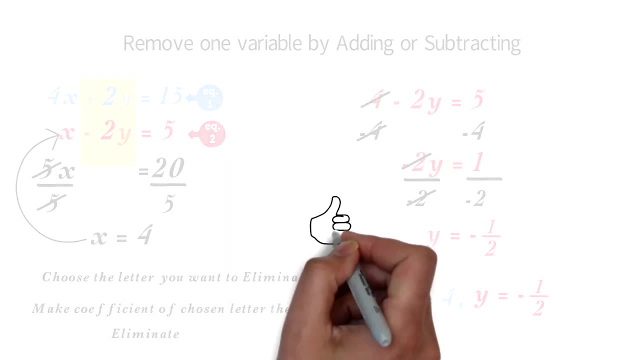 So we will have: y equals negative 1. Over 2.. So our final answer will be: x equals 4. And y equals negative 1 over 2.. Before we go to our next examples, we want you to do us a huge favor. 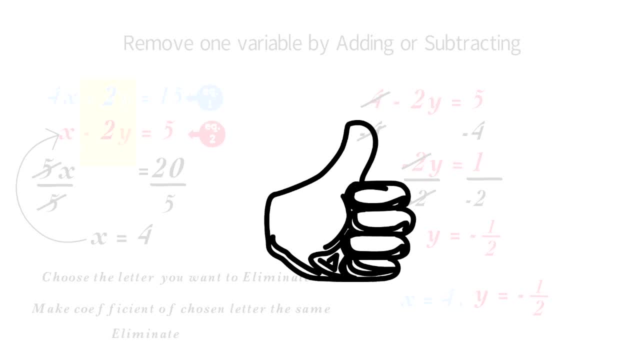 Smash the like button. We make these videos for you, so if we don't know you like them, there will be no reason to make more. Thank you. Let's look at example 2.. 1.- 1., 2., 3.. 4., 5., 6., 7., 8., 9., 10., 11., 12., 12., 13., 14., 15., 16., 17., 18. 19.. 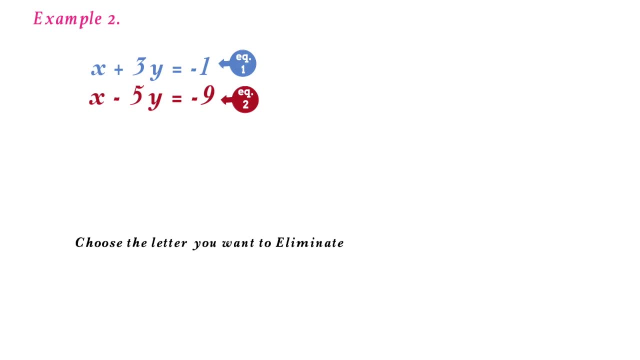 21., 22., 22., 23., 24., 25., 26., 27. 28.. the same coefficient. it will be best to choose that one because it will take care of step two. So here I will choose the x. Next, you want to make the coefficient the same. 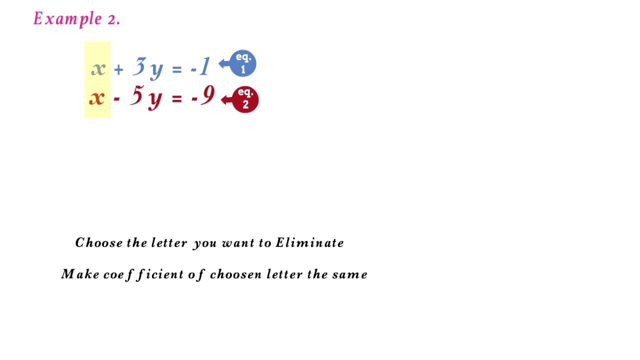 Here, the coefficient of the x are already the same, so there's nothing to do in this step. Remember, when you have no coefficient written, the coefficient is one. The next step is to eliminate the x values. Since both are positive, we can subtract the two equations so that the x value will be zero. 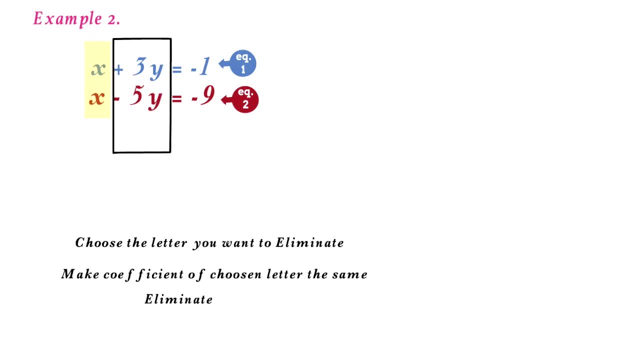 x minus x will be zero. 3y minus negative 5y equals 8y. We know that the minus negative is addition. The negative 1 minus negative 9 equals 8.. Now we have a simple equation we can easily solve: 8y equals 8.. 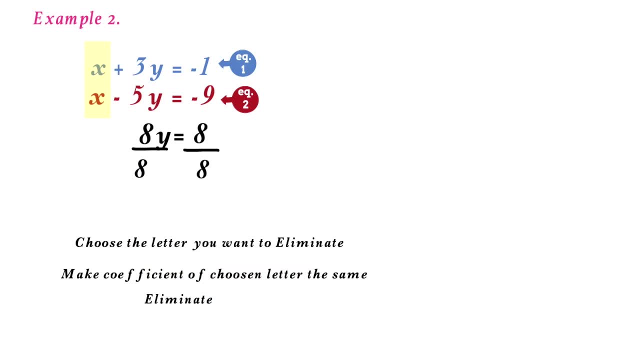 We solve this equation by dividing both sides by 8.. The 8 will cancel out. 8 divided by 8 equals 8.. 8 divided by 8 is 1.. So we have y equals 1.. To find the x value, just substitute y equals 1 into any of the equations and solve. 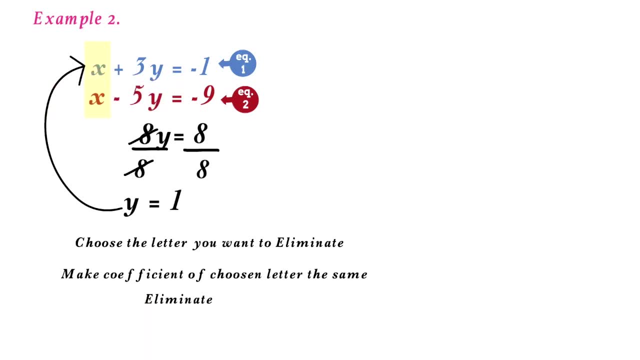 I will choose equation 1.. So I have x plus 3 times 1 equals negative 1.. Let's solve for x: 3 times 1 equals negative 1.. 3 times 1 is 3.. So we have x plus 3 equals negative 1.. 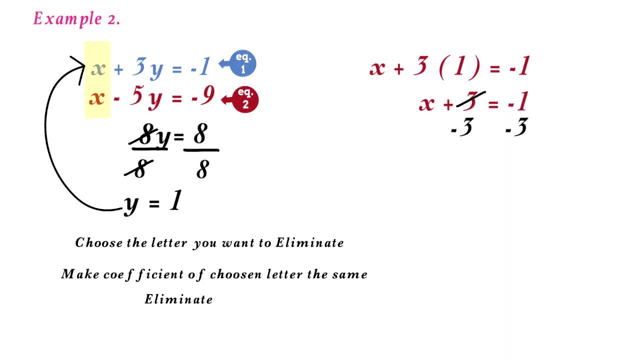 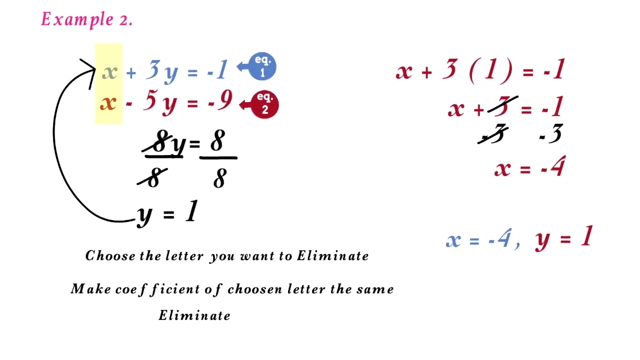 Subtract 3 from both sides, The 3 will cancel out Negative 1 minus 3 is negative 4.. So x equals negative 4.. Our final answer is therefore: x equals negative 4. And y equals 1.. Okay, we have looked at two examples in which one of the variables have the same coefficient in both. 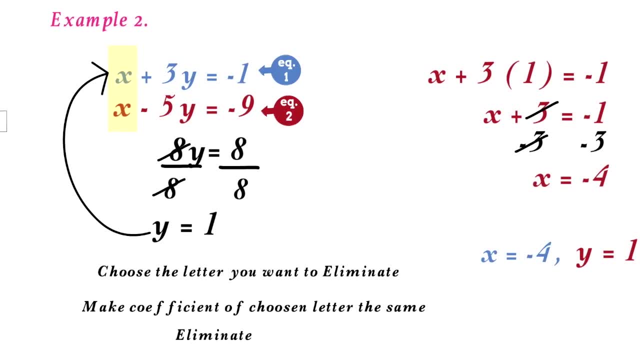 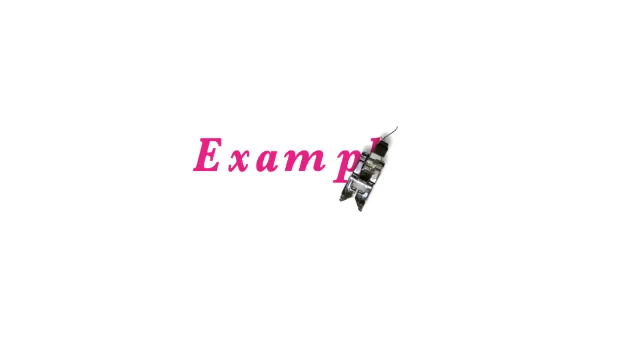 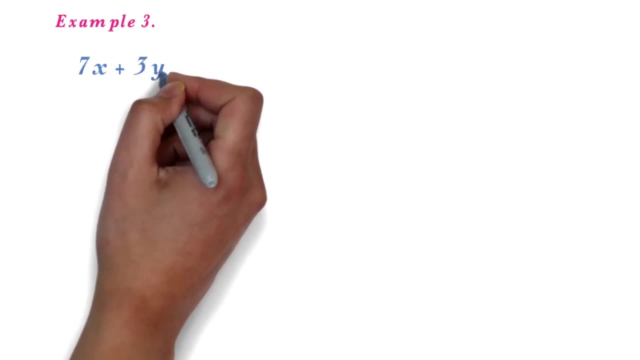 equations. Let's look at examples where we have to manipulate the coefficient before solving. Let's look at example 3.. We want to solve the simultaneous equations: 7x plus 3y equals negative 2. And negative 14x minus 9y equals negative 8.. 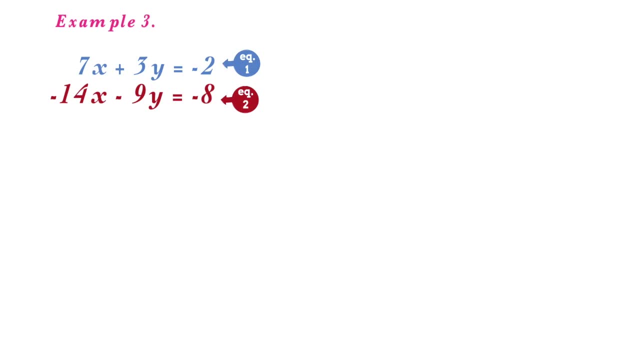 Let's call this equation 1 and this one equation 2.. The first step is to choose the letter you want to eliminate. It really doesn't matter which one you choose. I always try to choose the easier one. I will choose x. 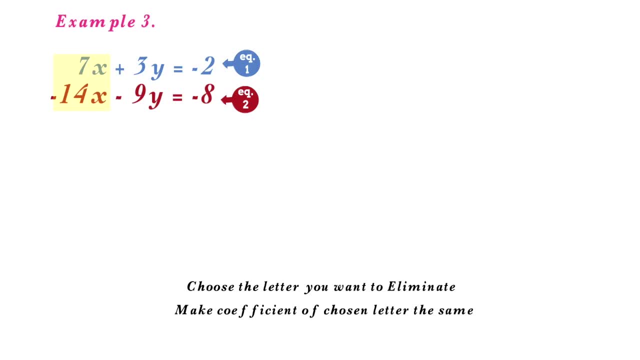 Next, you want to make the coefficient of the letter you want to eliminate. I will choose x letter. you want to eliminate the same? In the last two examples we looked at cases in which the coefficient of one of the letters is already the same. Here 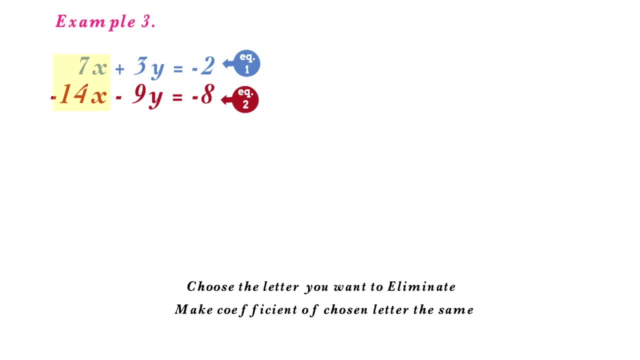 none of the coefficients are the same. So check if one of the coefficients is a multiple of the other. Here we see that 14 is a multiple of 7.. 7 times 2 will give us 14.. So we can multiply equation 1 by 2 so that we can make the. 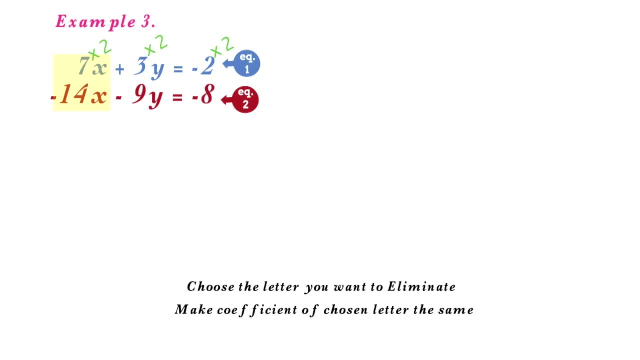 coefficient of the X the same. This will give us 14 X plus 6 Y equals negative 4.. We will call this equation 3.. The next step is to eliminate the X values. We will be using the equation 3 to eliminate the X values, So we will call. 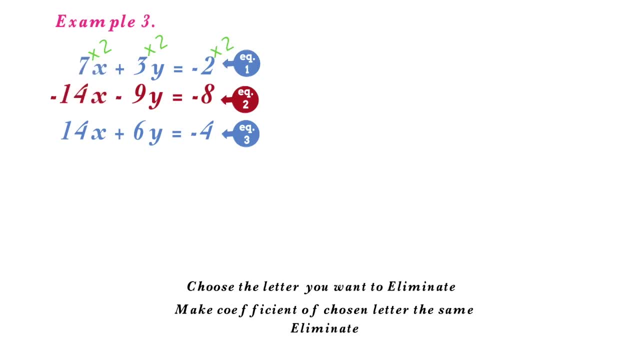 the equation 2.. The next step is to eliminate the X values We will be using in equation 2 and equation 3.. Since one is positive and the other is negative, we can add the two equations so that the x value will be 0.. 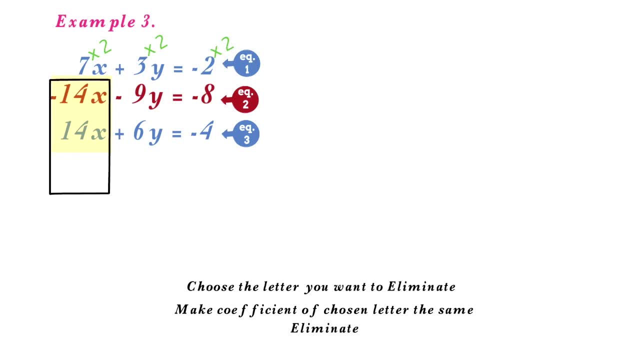 Negative 14x plus 14x equals 0.. Negative 9y plus 6y equals negative 3y. Then negative 8 plus negative 4 equals negative 12.. Now we have a simple equation we can easily solve. 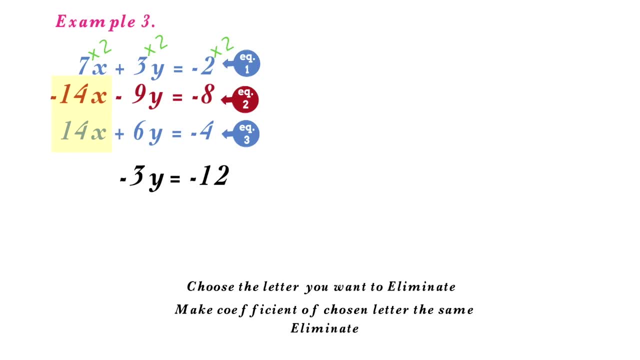 Negative 3y equals negative 12.. We solve this equation by dividing both sides by negative 3.. The negative 3 will cancel out Negative 12 divided by negative 3 equals negative 12.. Negative 3 is 4.. Therefore, y equals 4.. 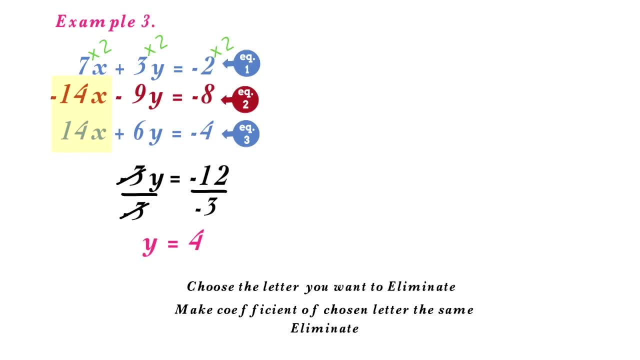 To find the x value, just substitute y equals 4 into any of the equations and solve. I will choose equation 1. 7x plus 3 times 4 equals negative. 2. Let's solve for x: 3 times 4 is negative 2.. 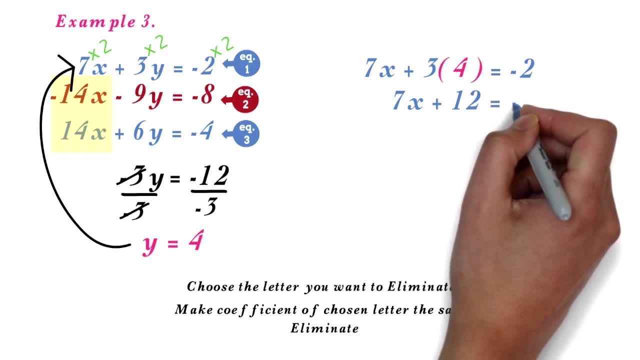 3 times 4 is negative. 2.. 3 times 4 is negative 2.. 3 times 4 is 12.. 28 times 8 is negative 2.. After figuring out the base, you will find out the yesterday's equation. 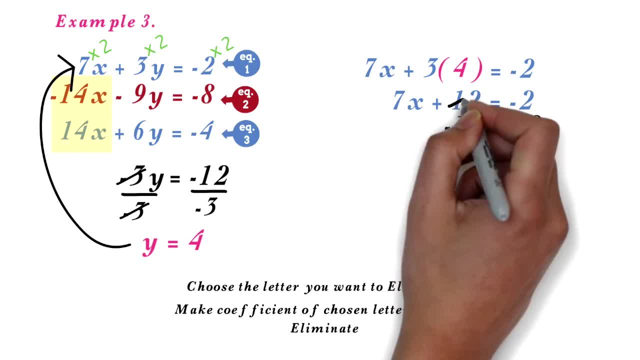 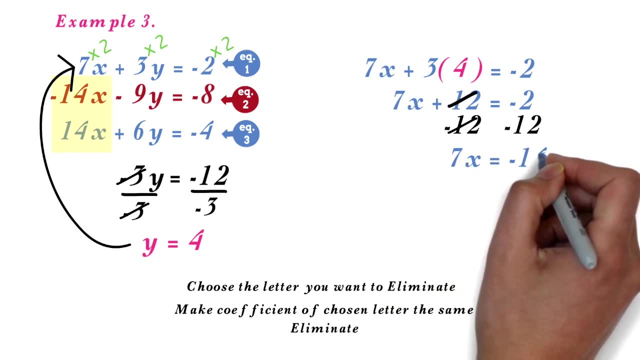 Subtract 12 from both sides, The 12 will cancel out Negative. 2 minus 12 equals negative 14.. Next we divide both sides by 7.. The 7 will cancel out Negative. 14 divided by 7 is negative 2.. 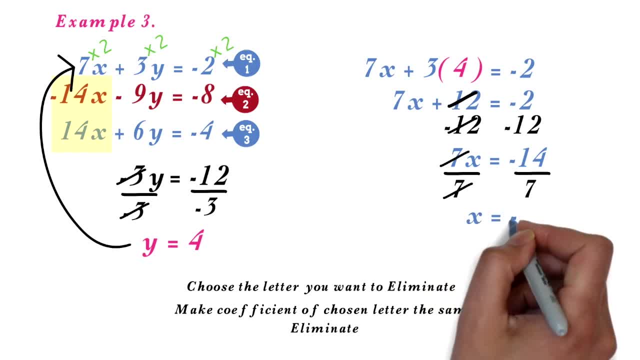 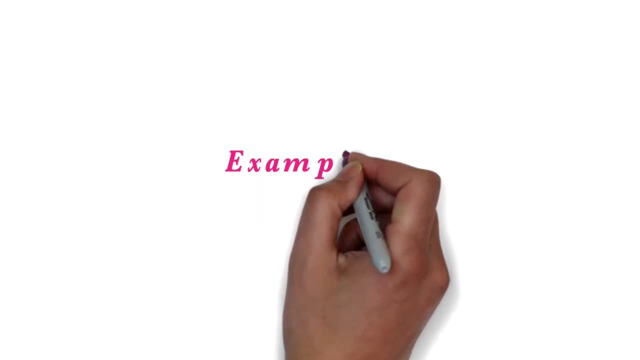 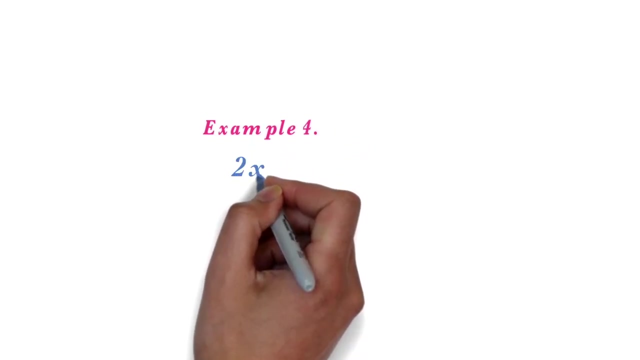 We are done by now. Therefore, x equals negative 2.. Our final answer is therefore: x equals negative 2 and y equals 4.. Let's take our last example, Example 4.. We want to solve the simultaneous equations: 2x plus 3y equals 8.. 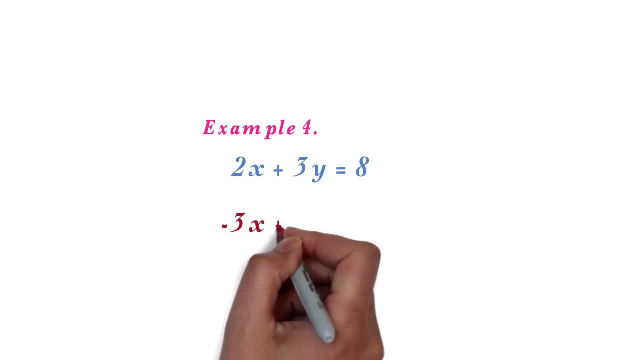 And negative 3x plus 4y equals 5.. Let's call this equation 1 and this equation 2.. The first step, as always, is to choose the letter you want to eliminate. It really doesn't matter which one you choose. 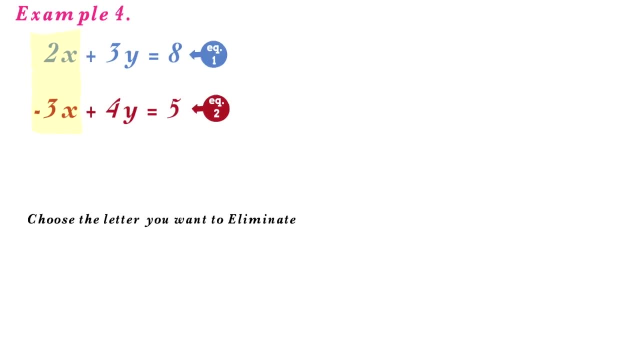 I will choose x. Next, you want to make the coefficient of the letter you want to eliminate. In this question, we see that none of the coefficients are the same And also none of the coefficients is a multiple of the other, So we will use the idea of cross-multiplying the coefficient. 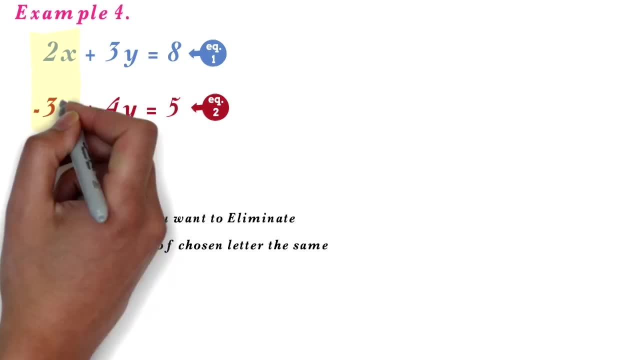 We will multiply equation 1 by the coefficient of the x in equation 2.. So we will multiply equation 1 by the coefficient of the x in equation 2.. By negative 3. The negative doesn't really matter, So you could have just multiplied it by 3.. 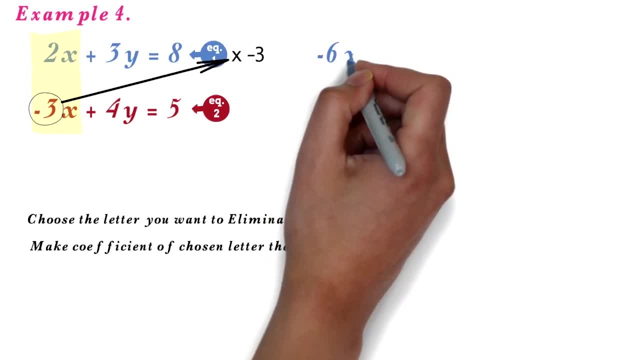 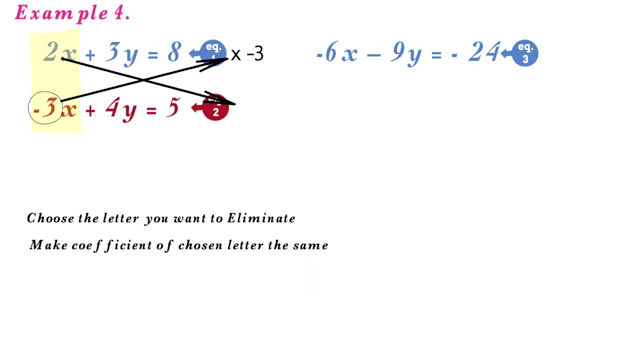 So we will get negative 6x minus 9y equals negative 24.. Let's call this equation 3.. We will then multiply equation 2 by the coefficient of the x. We will then add in the x in equation 1.. 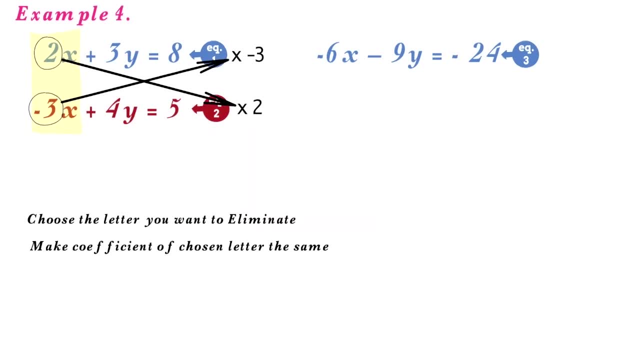 So we will multiply it by 2. So we have negative 6x plus 8y equals 10.. We will call this equation 4.. The next step is to eliminate the x values. We will be using equation 3 and equation 4.. 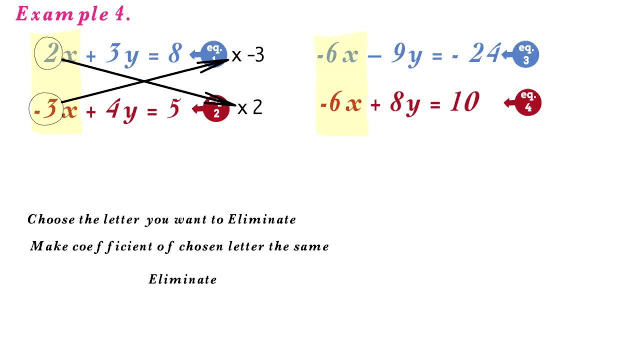 Since both are negative, we will call this equation 3.. both are negative. we can subtract the two equations so that the x value will be zero Negative. six x minus negative six x equals zero Negative nine y minus eight y equals negative seventeen y. Then negative twenty-four minus ten equals negative thirty-four. Now, 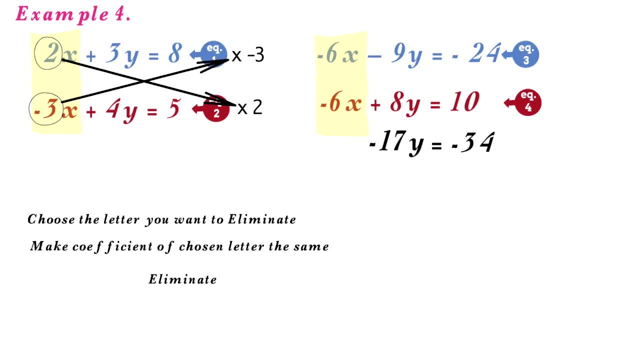 we have a simple equation we can easily solve: Negative seventeen. y equals negative thirty-four. We solve this equation by dividing both sides by negative seventeen. The negative seventeen will cancel out Negative thirty-four divided by negative seventeen is two. Therefore, y equals two. To find the: 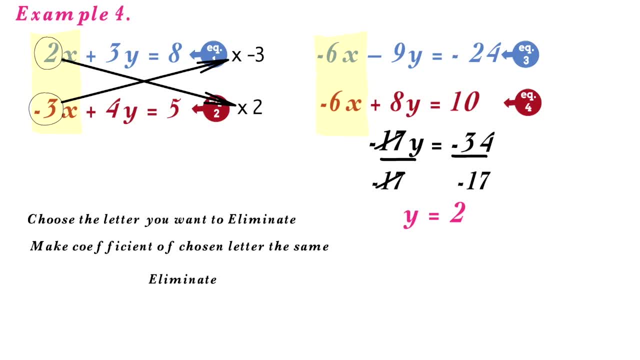 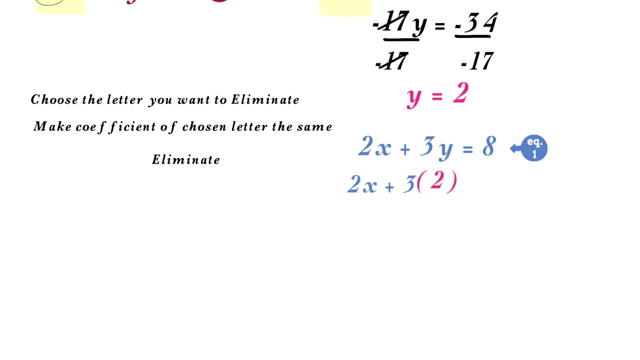 x value, just substitute y equals two into two. To find the x value, just substitute y equals two into two. To find the x value, just substitute y equals two into two. To find the x period, draw a figure b into any of the equations and solve. I chose equation one, Two x plus three times. two equals eight. clo今天 chúng ta l выбorrow straight out of the equation and solve it. Let's solve for x: Two, x plus three times two equals eight. Negatives three and twousing two equals six. Da Bitte einen neuen Minuske in positive пол und Countersprise. 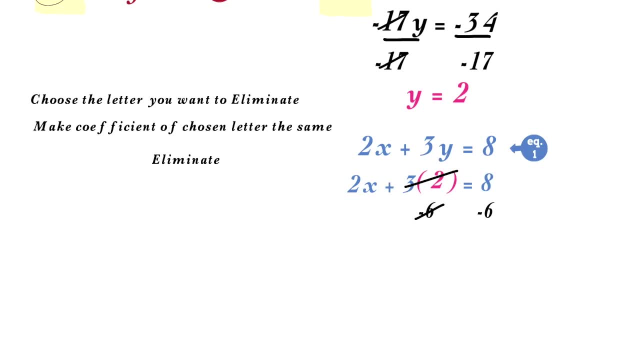 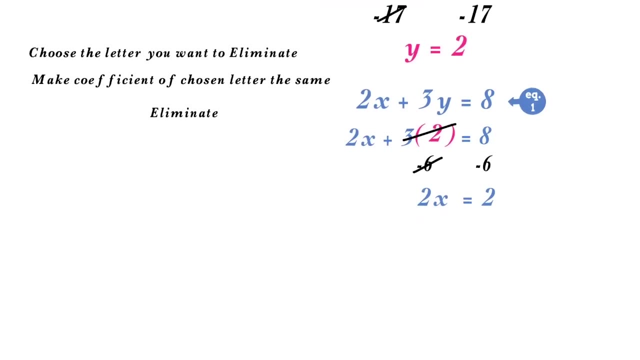 Three times two is six Debuten sechs von beiden Seiten. Das wird eine sehr große 모습. This will cancel out. 8 minus 6 equals 2.. Next we divide both sides by 2. The 2 will cancel. 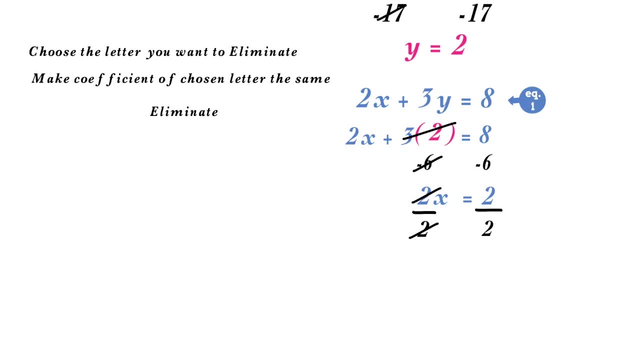 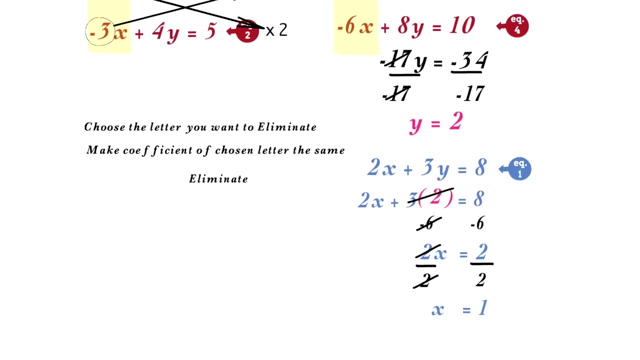 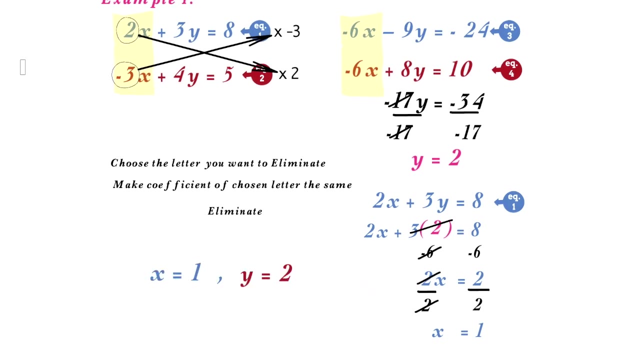 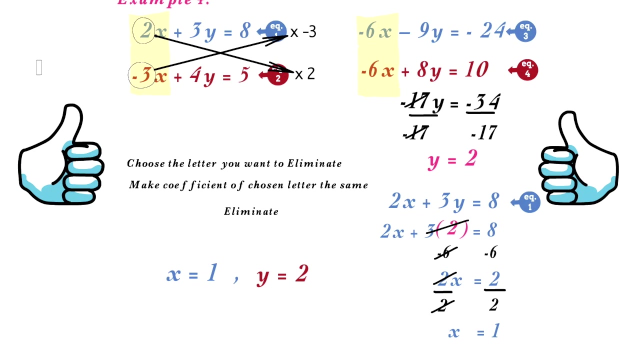 out: 2 divided by 2 is 1.. Therefore, x equals 1.. Our final answer is therefore x equals 1 and y equals 2.. Please smash the like button to show your support. if you haven't done that yet, We deeply appreciate it.